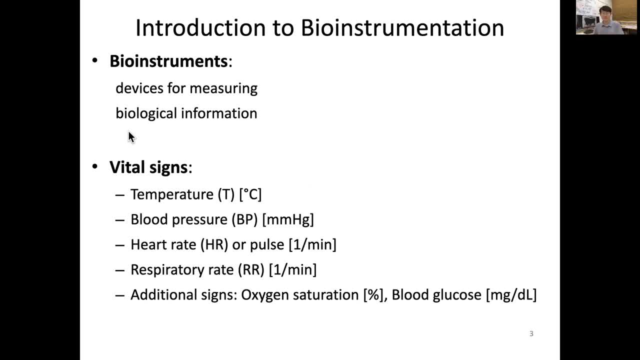 biological information, so it would be good to see when the patient went to doctor's office. So this is a modern hospital environment. when there are a patient you can see. on the back side there are like tools for measuring temperatures, blood pressure measurement and various number of instruments which 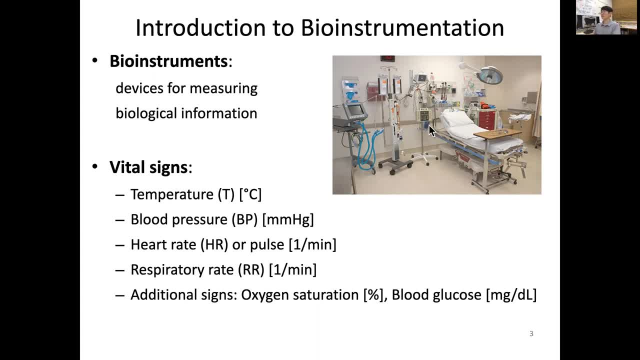 measures, vital signs of the patient. So vital signs are those crucial biological information which is very important for the integrity of the patient. So for example here, temperature- Of course we write it as T and Celsius, and the second is a blood pressure which is related to heart function and 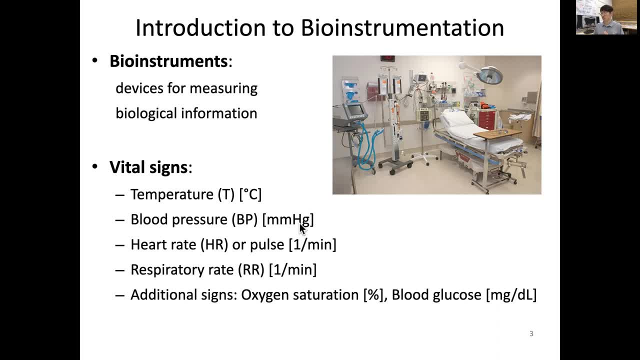 and the unit will be mm throughout. the unit CC number is heart rate, So all we write hr, or pulse, which is the number of heartbeats per minute, And another is the breathing rate or respiratory rate, So we call it RR and this is also the number. 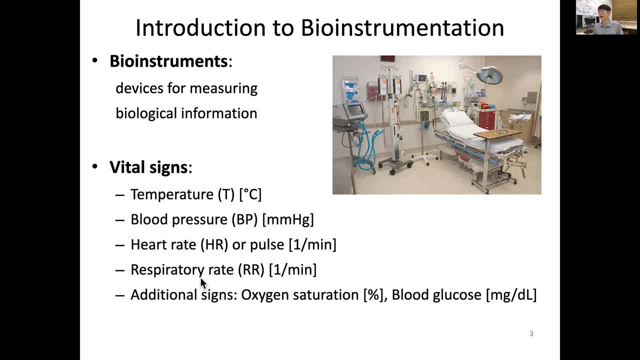 of breaths per minute. An additional science also. you know that the, the oxygen saturation in the blood, are important, so that as a percentage or a blood glucose is also important, which is the unit of milligram per deciliter. So for these vital signs we want to decide whether the patient is having. 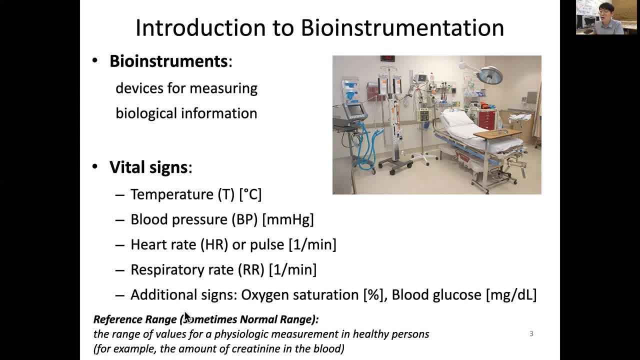 issues with this. So for that we define sometimes reference range or normal range. So these are the range of values for a physiological measurement in healthy persons, so that we can compare these ones with a patient Here, for example the amount of creatinine in the blood. So there are certain range of values for 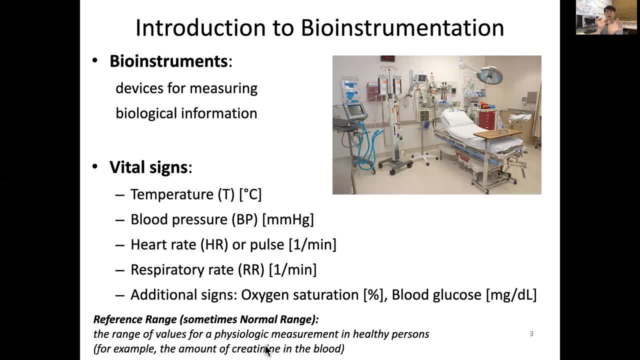 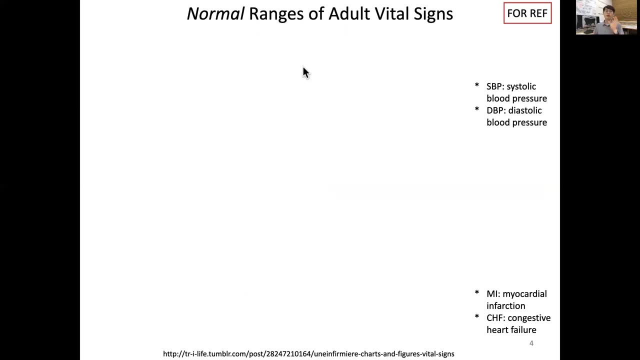 as a normal range. So when we measure the patient's creatinine in the blood we can say it may be abnormally high or abnormally low. So for that this is a reference information: Normal range of adult vital signs. So here is an. 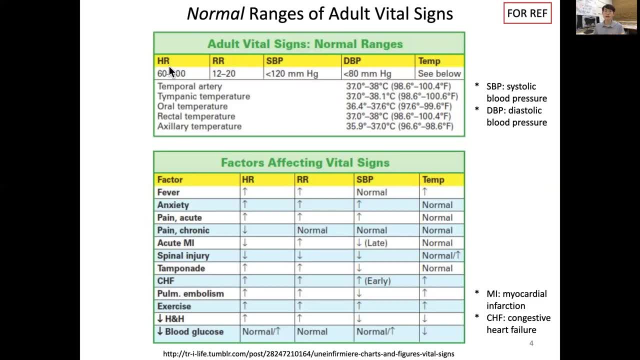 example Respiratory rate. So the heart beats is. the normal range is about 60 to 100 beats per minute. We consider it as a normal And respiratory rate. So the breathing is about 16 to about 20 times per minute as a normal And systolic blood pressure is. 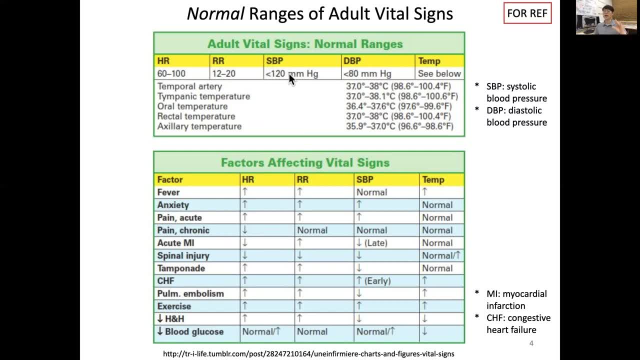 supposed to be less than 120 mmHg. If it's higher than 140, we consider 30 or 20 times higher blood pressure, And diastolic blood pressure is supposed to be lower than 80 mmHg And temperature depends on where we measure the 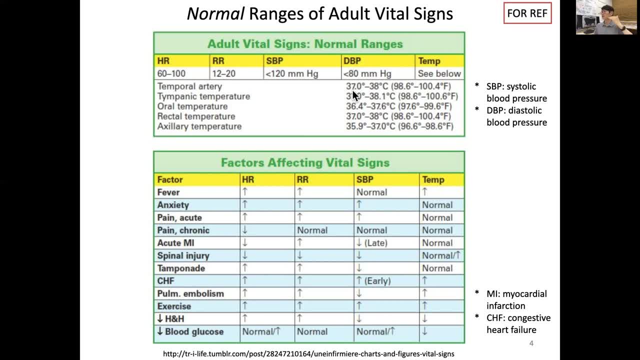 temperature. So, for example, temporal artery is like this range and tympanic temperature which is inside the ear, the tympanic membrane through that is this range And the oral temperature, rectal temperature and accelerated temperature. So that normal range is slightly different And in case of some, why these? 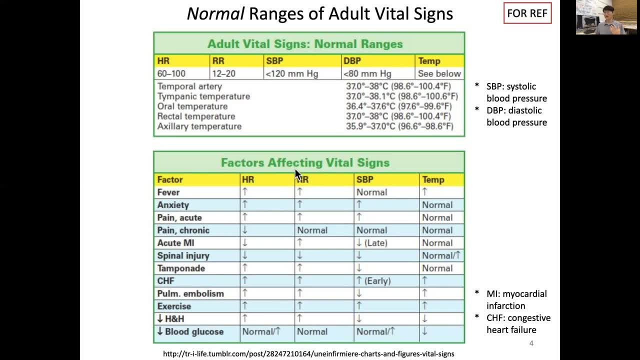 vital signs are important Because there is some indication in specific condition. For example, fever and anxiety makes the heart rate high, respiratory rate high and systolic blood pressure high. And another example: acute myocardial infarction. so myocardial infarction is like a heart. 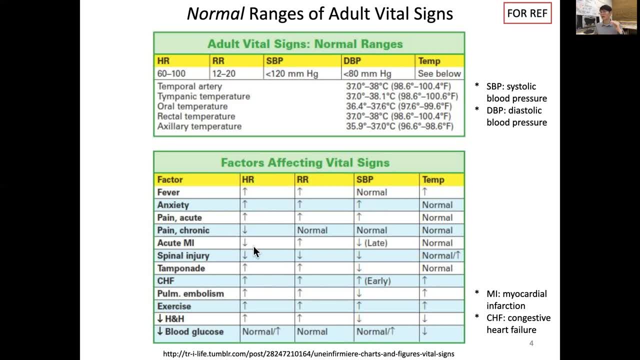 attack. so if it's acute and the heart cannot beat very well, so heart rate drops while breathing is higher to compensate the low oxygen and systolic blood pressure. because the function is as compromised, systolic blood pressure goes to late. so like this, there are a number of conditions. 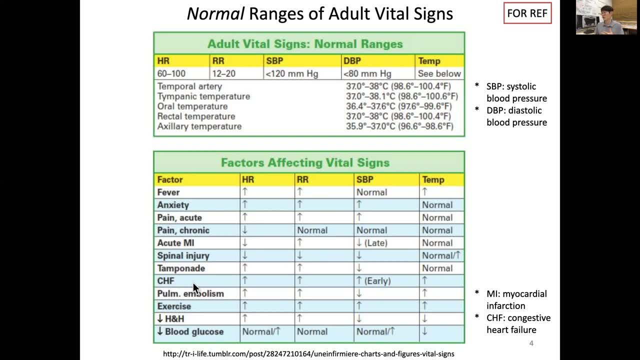 another example as a congestive heart failure, which means that the heart, it's a disease condition, that the heart is so weak that it cannot function to meet the body's normal demand and in that case the heart is trying to to. heart rate goes up, it's higher to compensate the heart rate and respiratory rate is also. 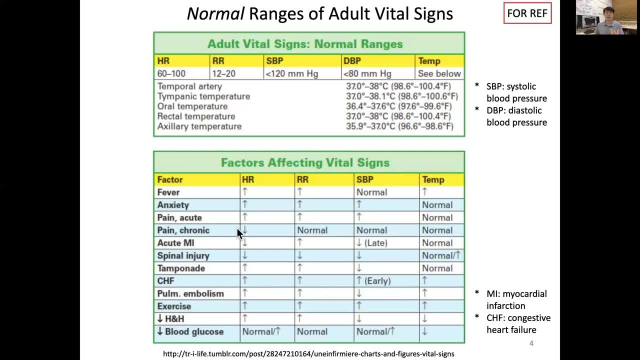 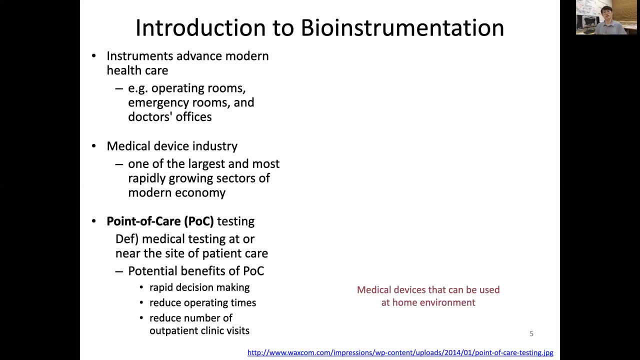 higher. so this is some kind of vital signs of heart failure. why it's important for understanding and measuring vital signs in and as a first line of a assessment for the patient. so now let's introduce bio instrumentation. so bio instruments are very important because they advance modern health care. so you, you see the operating rooms and 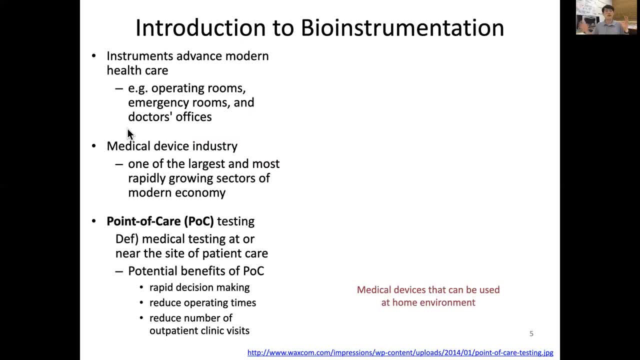 emergency rooms and doctor offices now filled with these bio instruments. because of that, the medical device industry is one of the largest and first growing sectors of modern economy, so for that there is a tendency that these are bulky, a very costly instruments inside a clinic or doctor's office and that tend to be smaller and portable. and 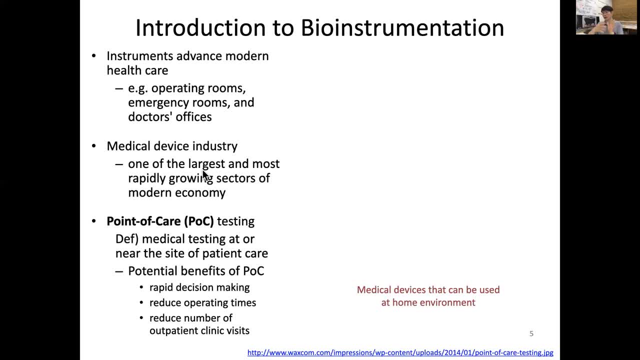 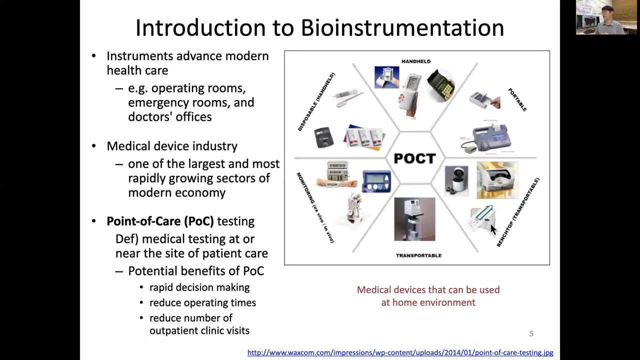 and it's available, lower cost to more like, like at home. so that is we call as a point of care, or POC testing, which means the medical testing at or near the side of patient care, like make patients home. so so let me show an example of 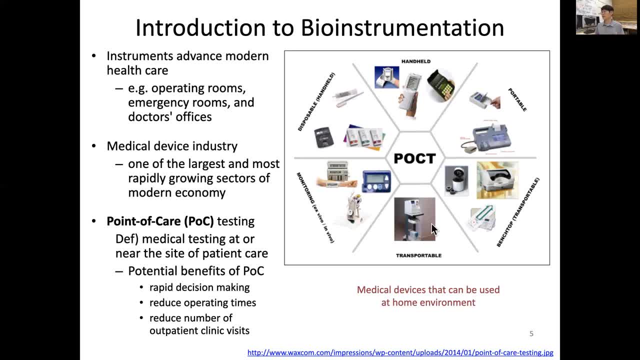 point-of-care testing device, which is now more transportable, and monitoring device for blood pressure- now it gets smaller and cheaper, so even a home can have it- and disposable handheld device, for example testing pregnancy. it's a nice, simple kit. nowadays it's a disposable and handheld device for for. 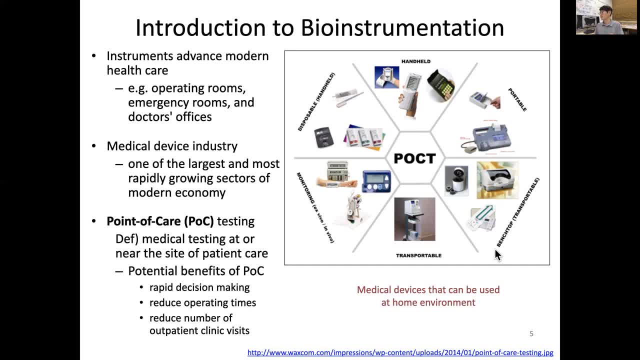 such as glucose monitoring device and bench-top device, so medical in devices. now they can be used at home environment. so why is it useful in that case? the benefits are many and, for example, the patient can make a rapid decision-making- of course it's this has to be dealt with a physician as well, and also operation times will be reduced. and 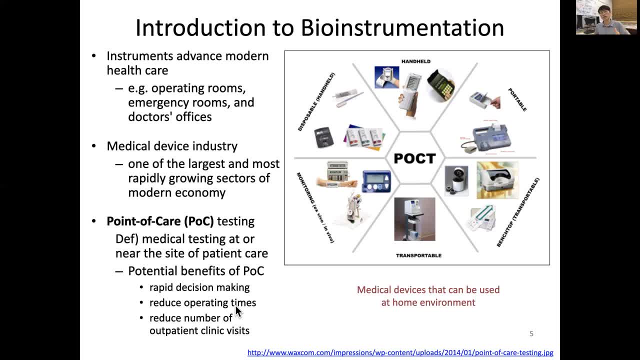 also the patient will generally find沒有 anestesia, no dedicatedpek学者, no, as losses then Harrison. and so another key use is for patient work. the patient is not accused for drugs, occupation, bizarreness of medical reasons, but also need to visit the clinic or hospital. so as the outpatient clinic visits will be, 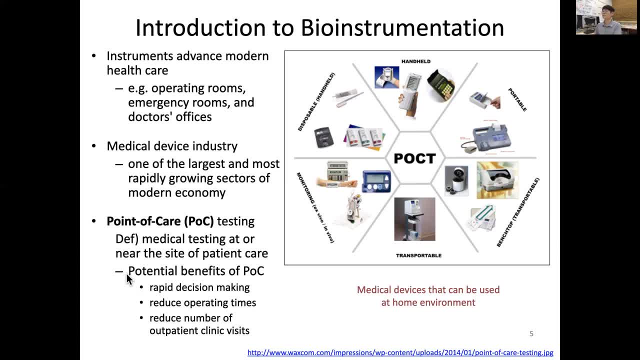 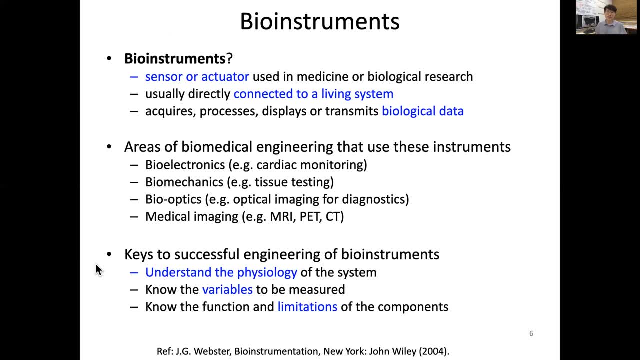 reduced So it's more convenient for the patient. So bio-instruments are like we can define as a sensors or actuators that is used in medicine or biological research Because of the bio on the instruments, so it actually uses directly, measures or connect it to a living system, and that 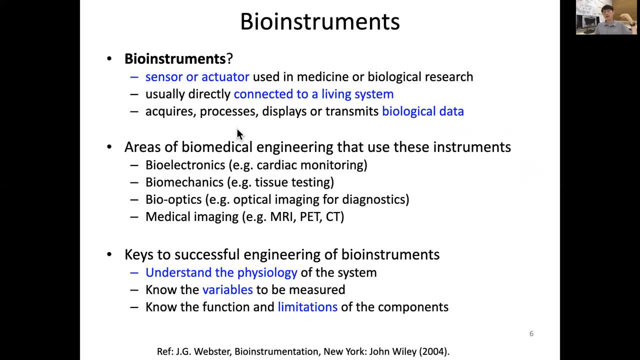 it acquires and processes and displays and transmits the biological data. So areas of biomedical engineering that uses these instruments are many. So, for example, bioelectronics- and good example is cardiac monitoring or ECG, EKG monitoring device- and biomechanics, which 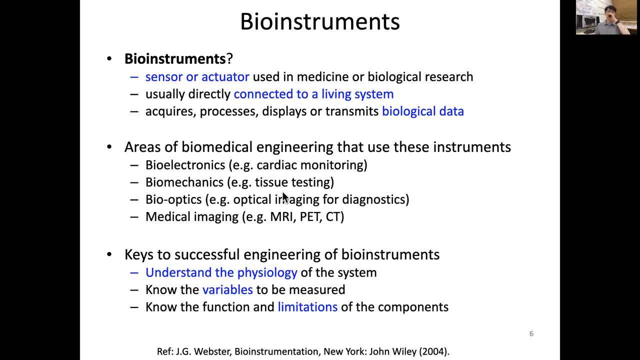 measures, for example tissue testing or, like long respiratory function tests. Another example is bio-optics, which is the optical imaging for disease diagnostics. A good example is an endoscopy optical endoscope, And medical imaging is also another area of using this instrument, such as MRI. 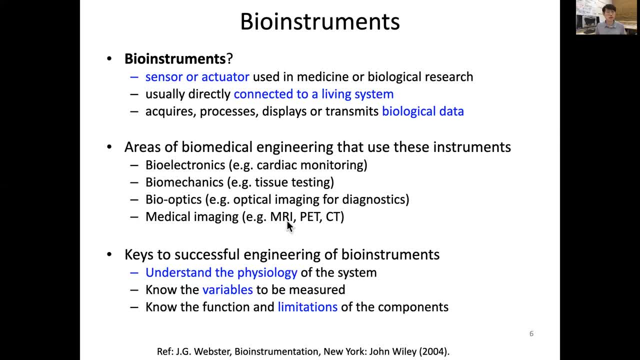 magnetic resonance imaging, cat positron emission tomography and CT, which is x-ray computed tomography, And these are like kind of instruments. So for the keys to successful engineering of bio instruments, where we first need to understand the physiology of the system, the biological system or the patient. 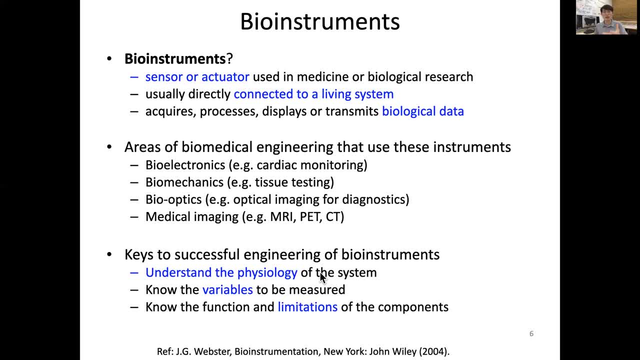 and the pathophysiology, the physiology of the diseased organs or function of the system and for instrument. we have to know the variables to be measured and also knowing the function of the components of instruments and also, very importantly, the limitation of the instruments, for example, the range of values which is 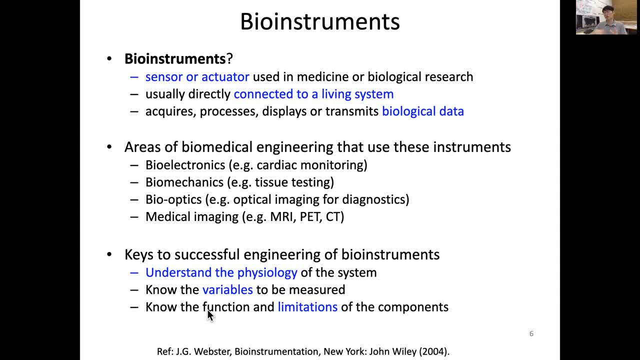 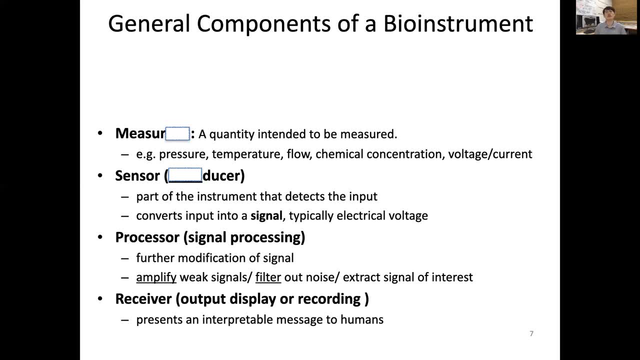 reliably measurable by the instrument you have to know for this. so now let's discuss about general component of bio instruments. so here it's a diagram showing. so we have an input. so which is we call measure on. so this is a measurement, is a quantity that is intended to be measured, so that's a. 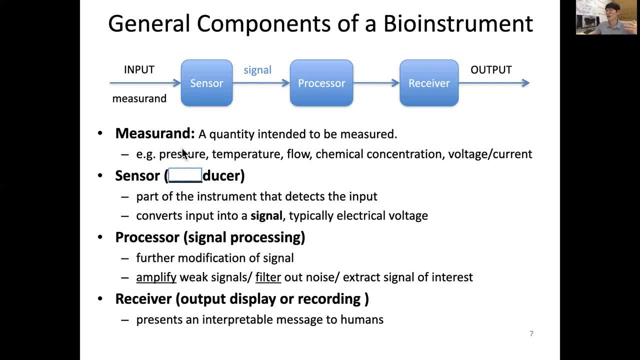 measure. For example, we want to measure blood pressure, patient temperature, blood flow, chemical concentration or voltage current, And those are the measurands and that can be measured by sensor. So sensor is a part of instrument that detects the input and usually converts into a signal. 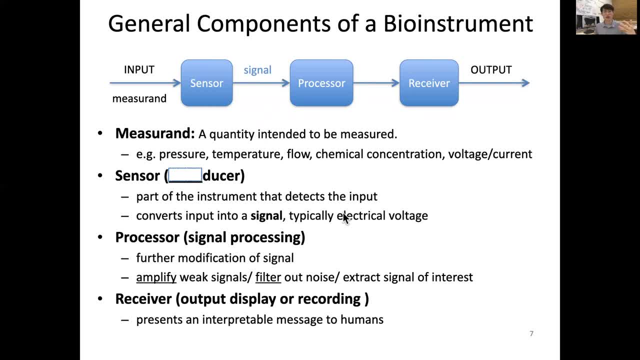 Signals are now mostly electrical voltage here. So input can be a various physical entity or electrical entity that converts into electrical voltage. So sensor is on the other way. it's called as transducer. So you remember, in cell signaling pathway there is a signal transduction pathway we call 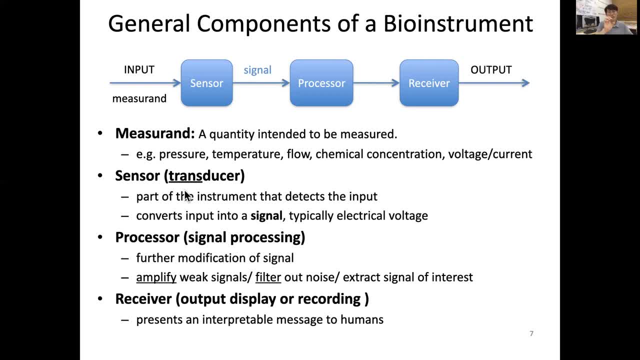 Because transduce means a converting voltage, One type of signal to another type of information. So sensor is a transducer. Now you convert it into a raw signal. Then there needs a processing for the raw signal. So further modification of the signal, because many times the signals are so weak that you need to amplify the signal. 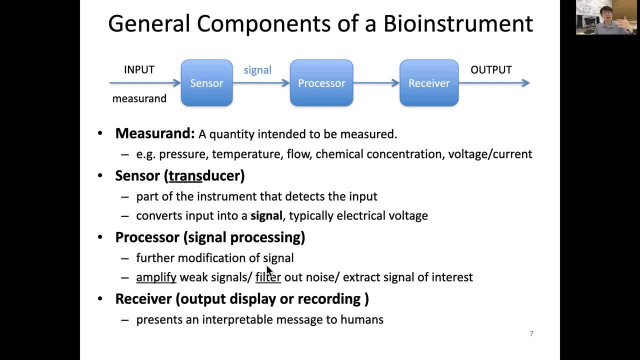 Also at the same time. signals usually comes with a noise So you have to sometimes condition Filtering out the noise. And signals there are, like your interest, signal of interest, you can extract from the signal. So all these collectively as we call signal processing.